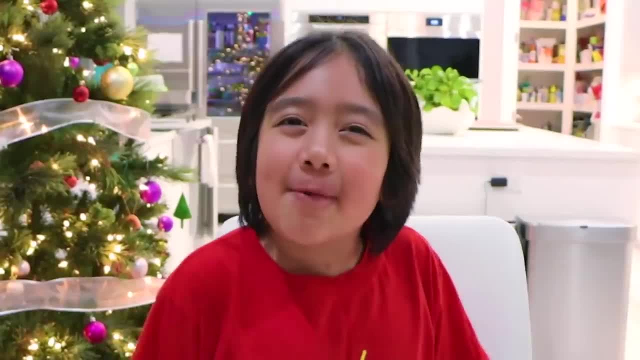 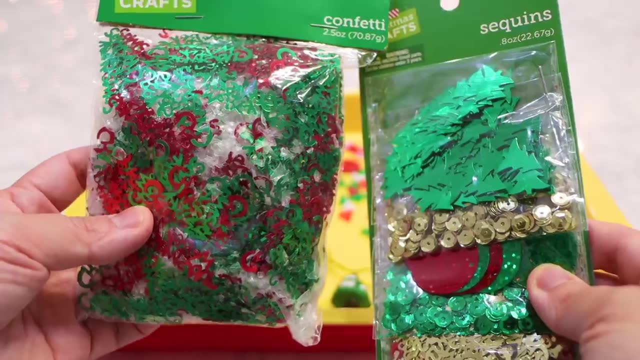 But first here's how to make it yourself. Take it away, Mommy. Roll the clip. The first thing to do is gather all of your favorite holiday things. I also have some confetti and some sequins, and you can add in some fun glitter. 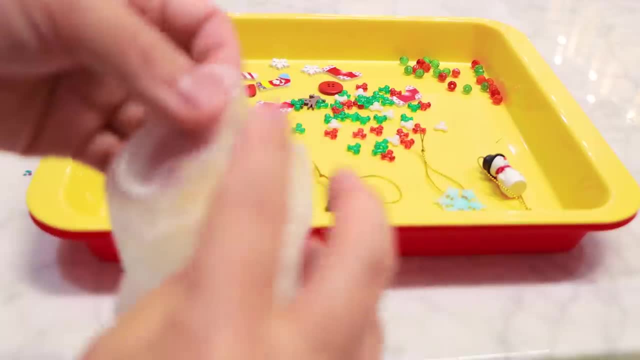 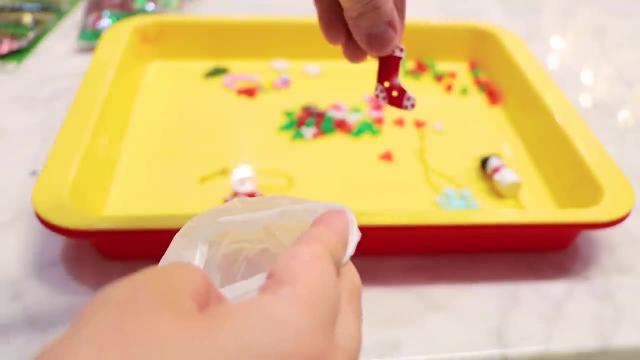 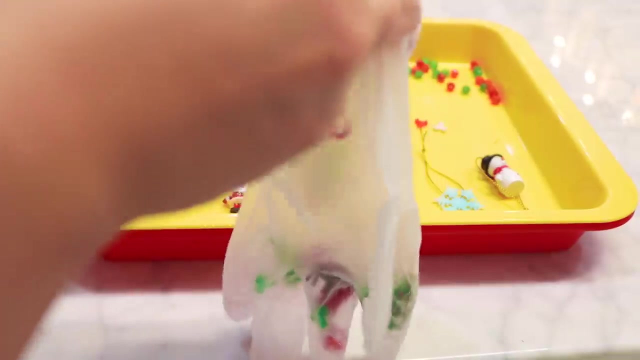 Next, grab a pair of gloves and then just put in your favorite things. Here I'm gonna put in a Christmas tree, some other fun things Stocking little cute reindeer, some fun Christmas patterns. Put it all in here, Some glitter. 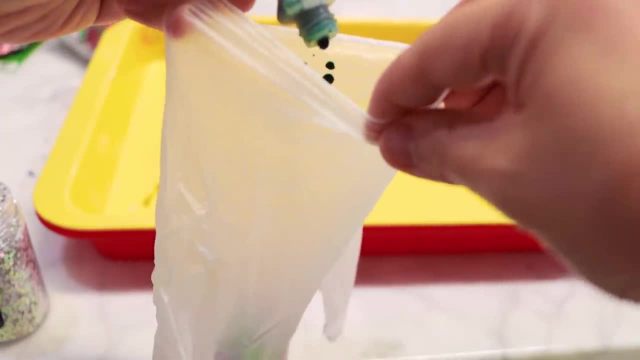 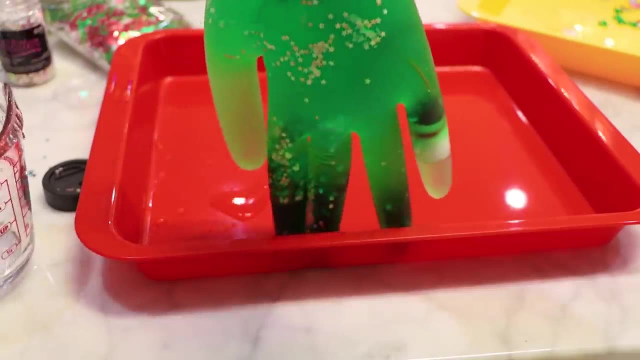 Then add in a few drops of food coloring. I'm gonna use green. Drop it in there. Then fill the glove up with some water. Fill it up three fourths of the way. Once you're done, tie it with a rubber band. 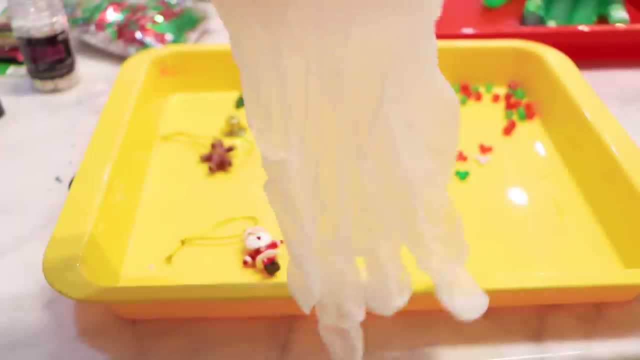 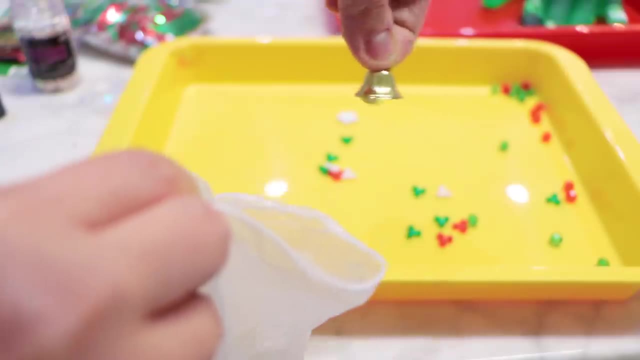 Whee. Okay, here's mine First hand. Okay for my second glove I'm gonna grab all this real cute. Hi Santa Claus, He goes into the glove, Cute little Bill Into the glove. Some fun Christmas trees. 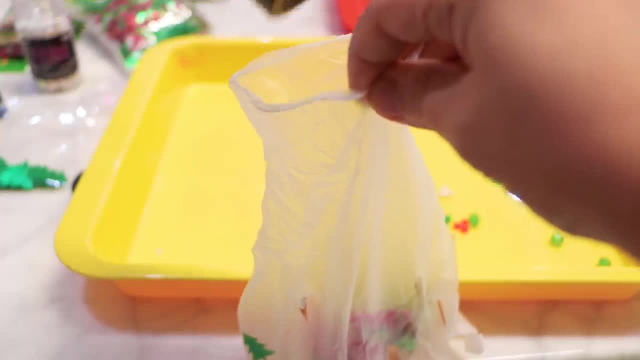 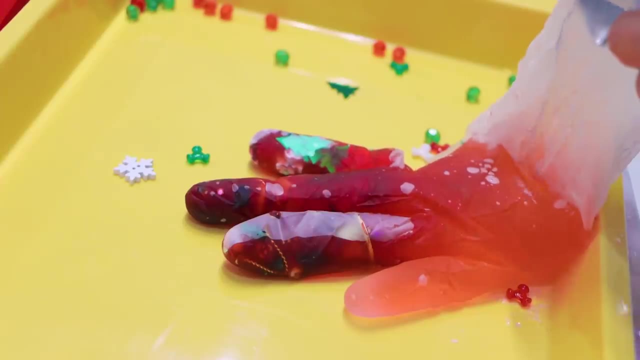 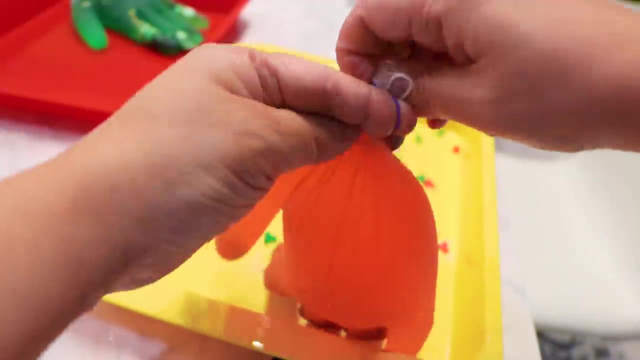 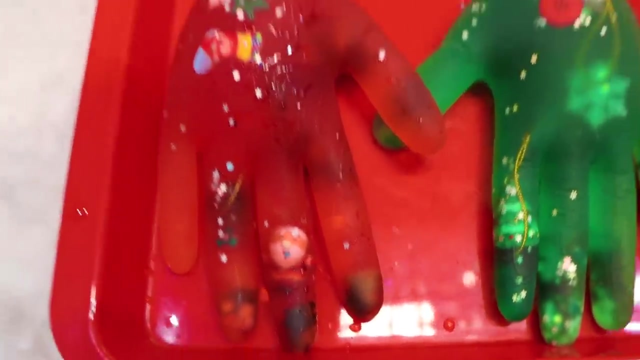 Some Christmas words, Then some fun glitter- Who doesn't like glitter? Then a few drops of red food coloring. Then add water. Once you're three, fourths done, Tie it with a rubber band. Okay, there's my red one. Look, I see Santa Claus. Do you guys see it? 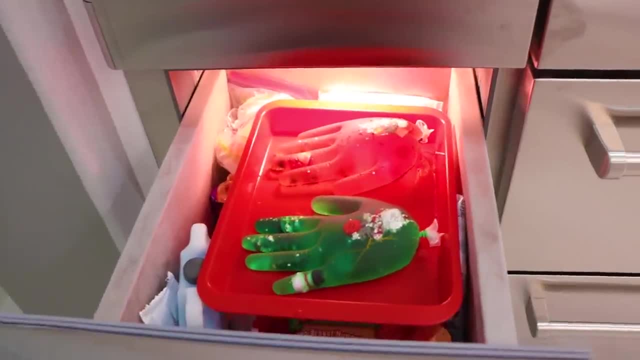 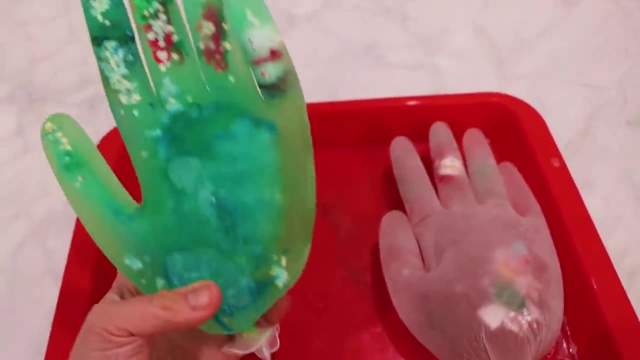 Once you're done, just put it in the freezer. There it is, I put it in the freezer. I'm gonna keep it overnight. Once it comes out here, it's all frozen. Do you guys see it? It's rock solid, hard. 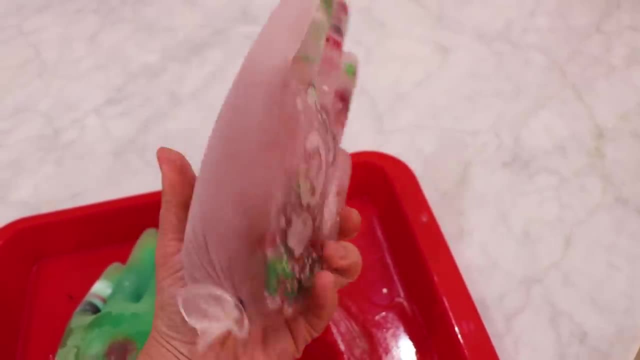 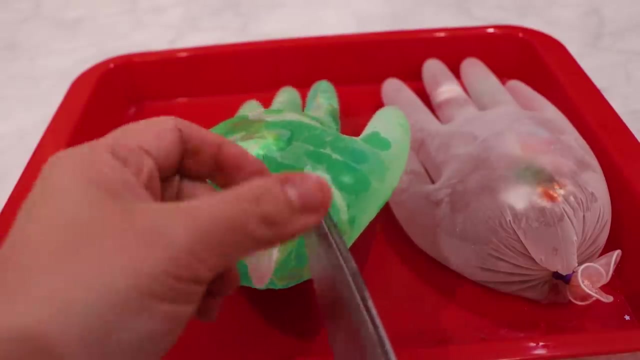 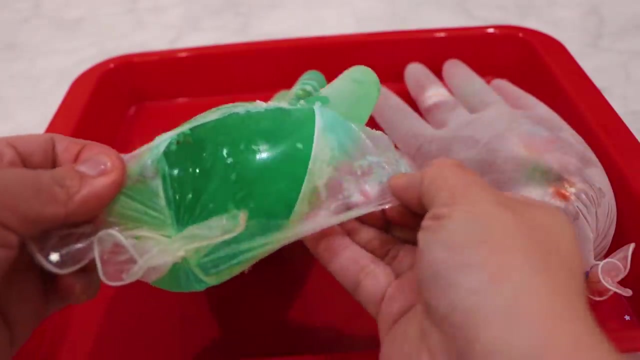 The red didn't stay very well. Should've added more red food coloring, But it comes out pretty good. Do you guys see Santa right there? Next, open up the rubber band and then cut And Pew. Be very careful of the fingers and thumb. 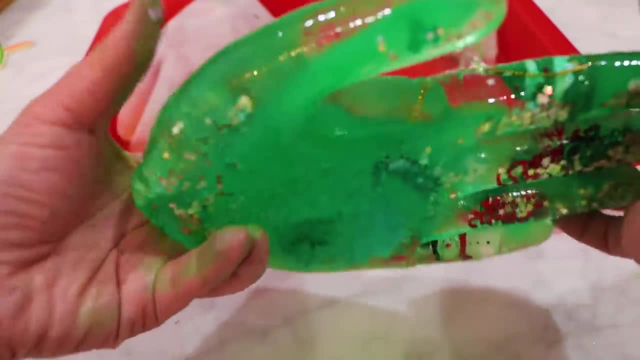 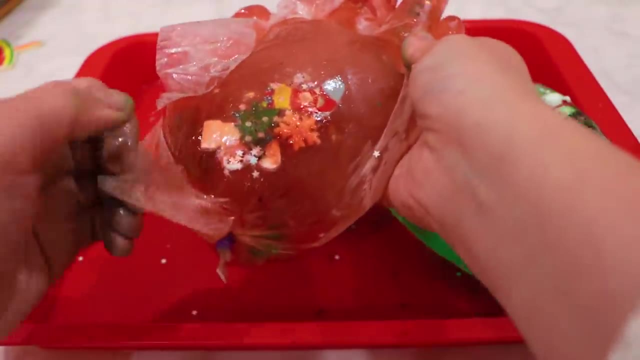 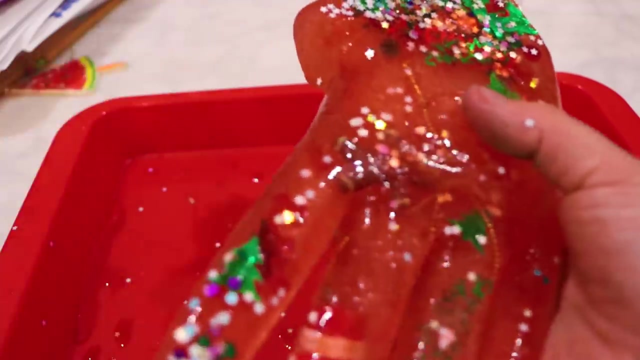 Once you're done, you'll have something like this: Isn't that cool? Look, be a snowman. Okay, here's the other one. Just pew And cut away. Look, there's Santa. Okay, and it looks like this. But guys, look, I broke off the thumb, Oh no. 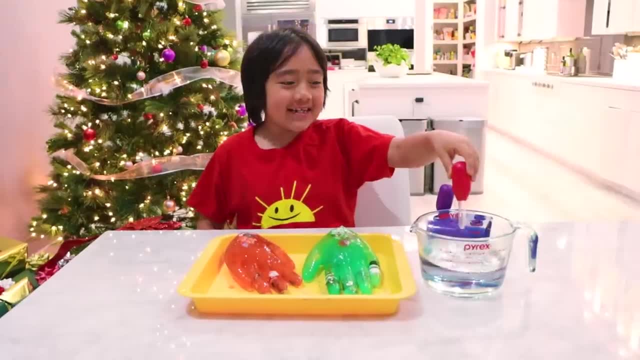 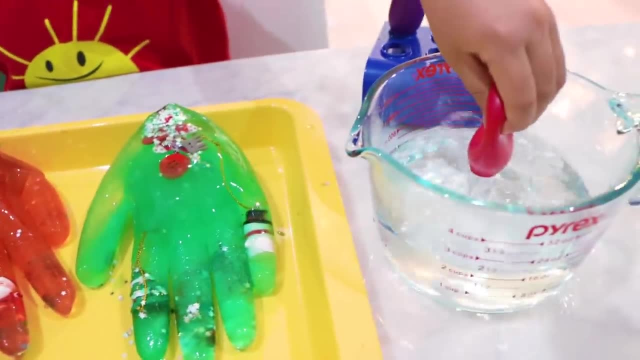 So okay, it's so fun. Look, there's Santa. Okay, let's get started. I'm gonna try to melt it with some warm water. It's working a little bit. Wait, wait, I can feel the objects. It's working. 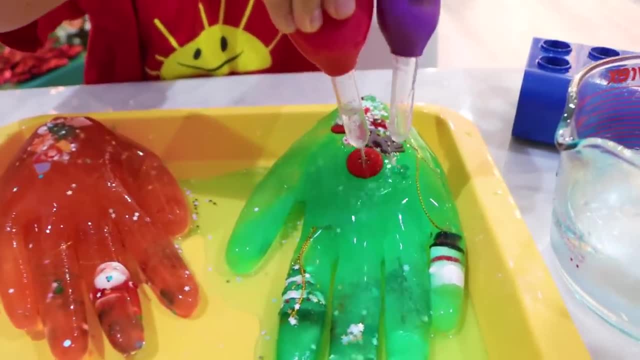 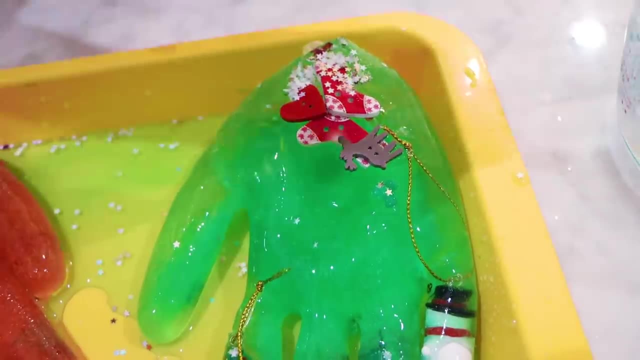 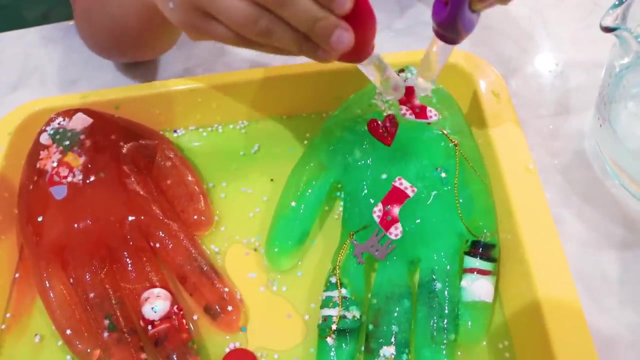 Okay, we're good. Okay, Did I get the button out? I got the button out. There you go, And there, I think this time I'll be able to free something. Oh wait, I freed a. I freed socks. 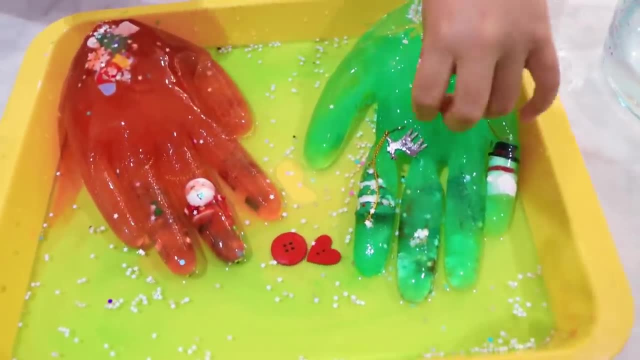 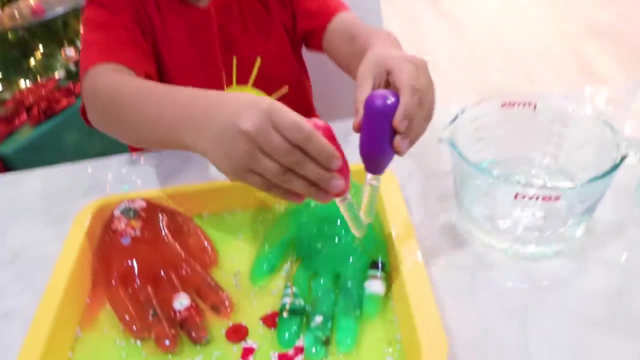 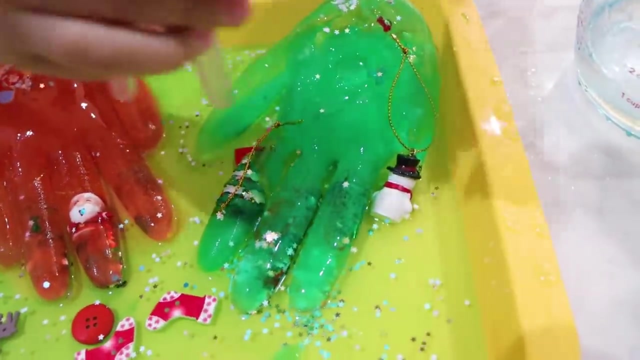 And a heart, Heart And socks And a deer. Oh, and another sock. Don't worry, snowman, I'm coming for you. I think I have to put all the water in one spot. I think the snowman's out. 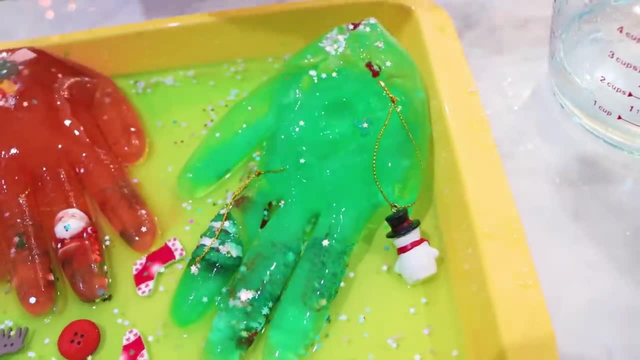 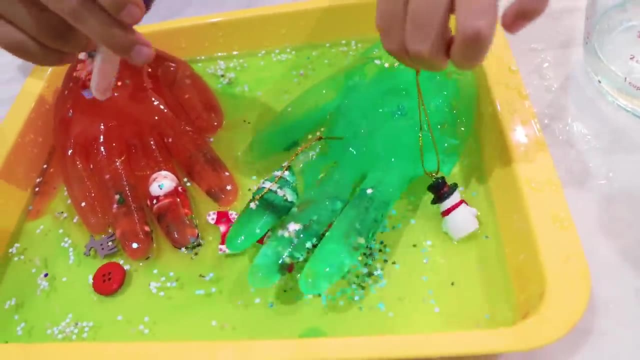 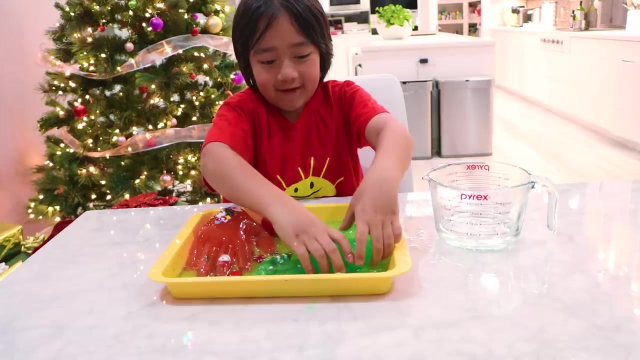 Oh oh No, there's a chain. I gotta get the chain out. Oh oh, oh. yeah, I think I got him out. Oh oh, oh, Got him out. Yes, Okay, guys, I'm gonna try to pick it up. 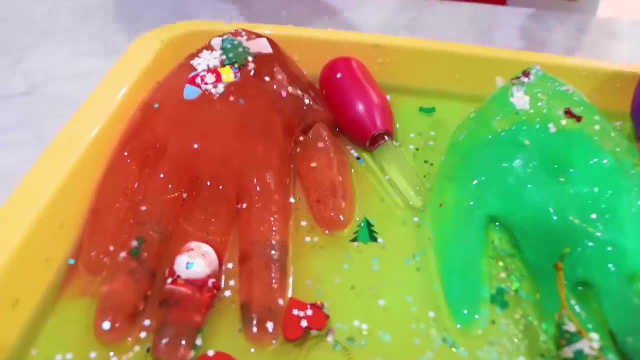 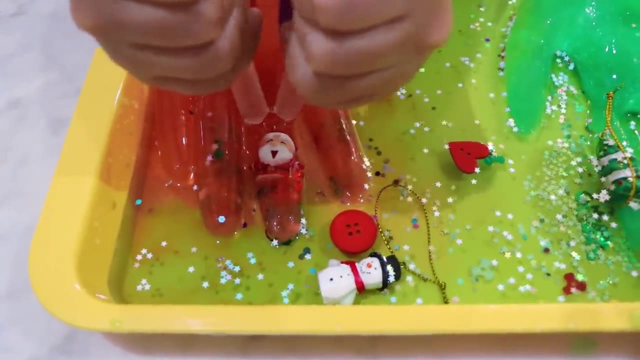 Oh, it's super cold and it's missing a pinky. Ah, This one's also missing a thumb. Okay, Santa, I'm gonna try to rescue you now If I put all of the horse right here. Oh, there's another golden chain. 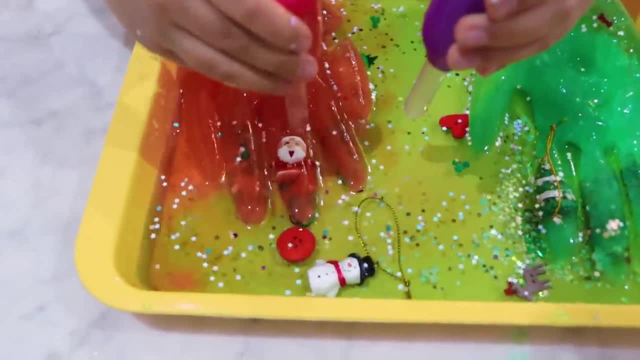 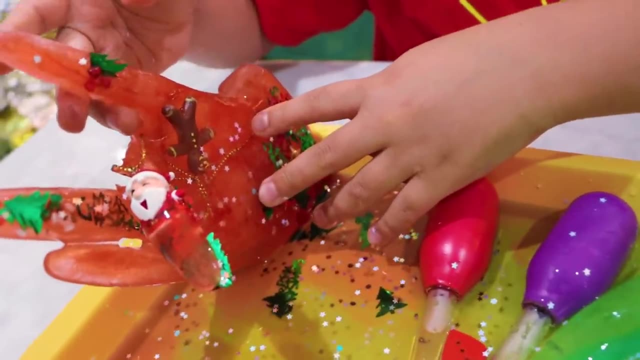 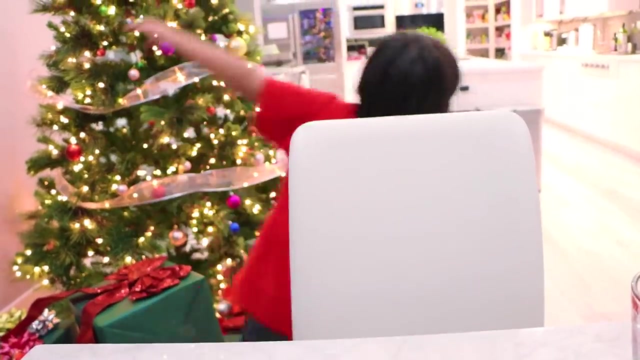 No, Where does the golden chain lead to, Guys? the chain is super long. It's all the way up to here. What do I do now? I have an idea: I'm gonna go get a mallet, guys. Okay, guys, I got two of them. 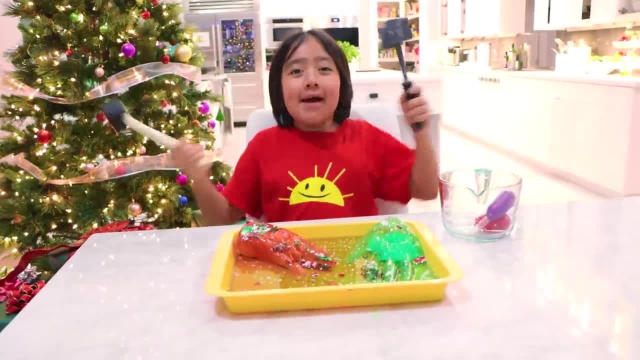 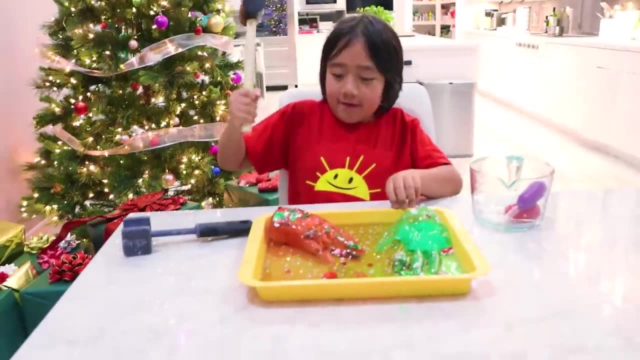 But remember to ask your parents for permission, because my mom said: yes, Right, Mommy, Yep, Okay, let's try this one first. I think that one will be stronger. Whoa, whoa, it's working, it's working.